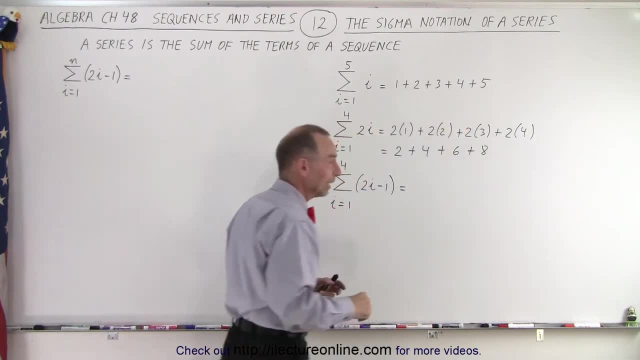 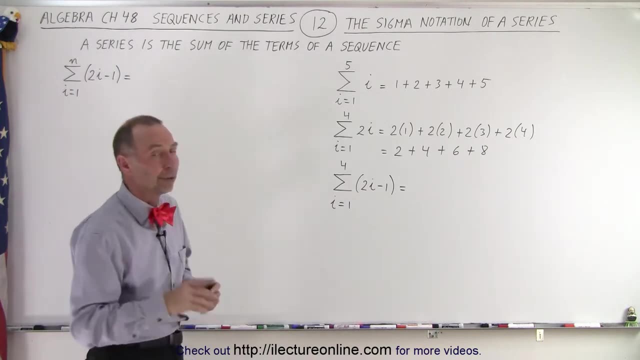 we could write it as one plus two plus three, plus four plus five. but what if we have an infinite series? We can't sit there forever. just add up all the terms We need to write in a compact form. and to do that, we have this symbol right here, which is the Greek letter sigma. And here we 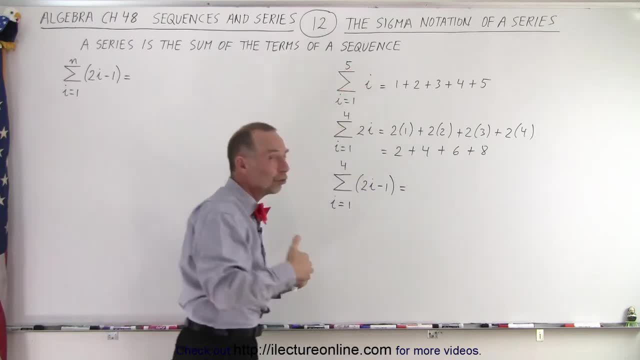 write when i goes from one to five and i goes up in integer format, so i will become one, then two, then three, then four, then five. This is the upper limit of the number i, starting from the lower limit, And here we have the sum of i's when they go from one to five, So when i is one. 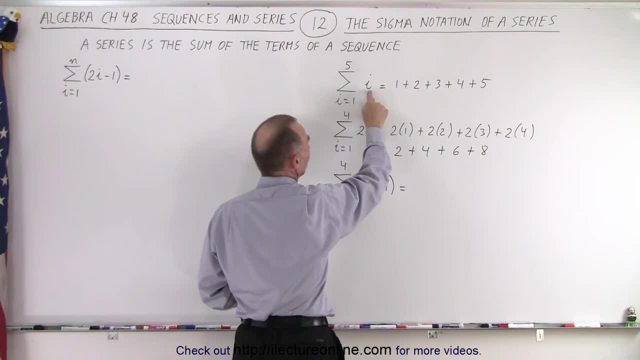 we get a one. When i is two, we get a two. When i is three, we get a three. When i is four, we get a four, And when i becomes five, we get a five. Why don't we go beyond five? Because the upper limit 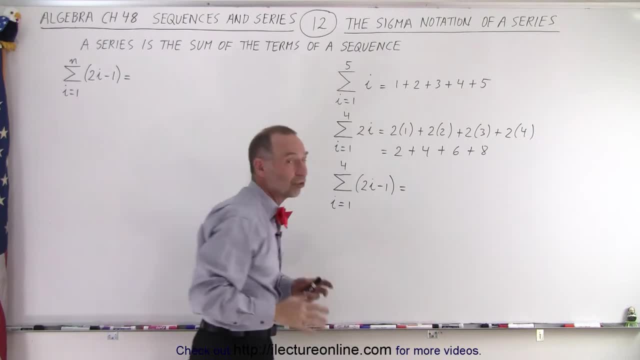 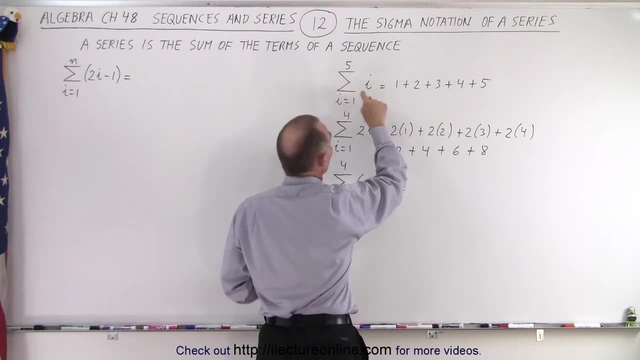 for i is five. Why do we start at one? Because the lower limit starts at one. it goes up like an integer And then we simply write the sum. This simply means the sum of all the i's going from one to five. That means one plus two plus three, plus four plus five. So this can be written in a 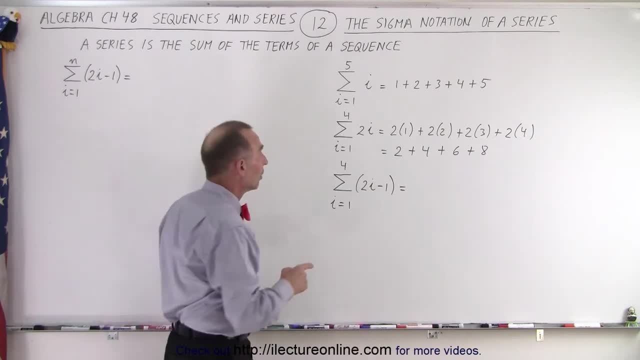 compact form like this. What if we write it like this: The sum from i going from one to four. so the upper limit here is four of two i. So each time we plug in the value for i, i will become one, then it will become two, then it will become three, then it will become four. We stop at four. 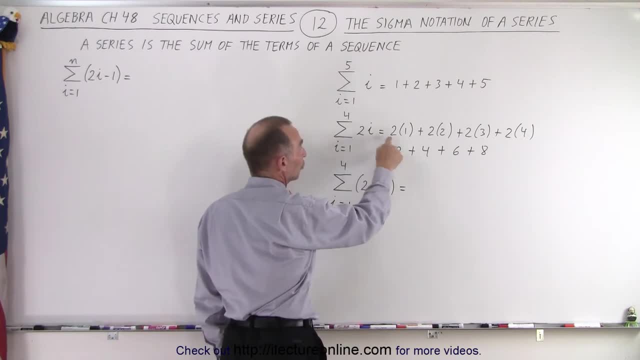 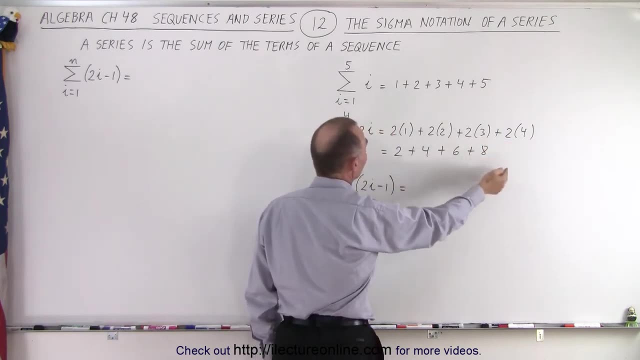 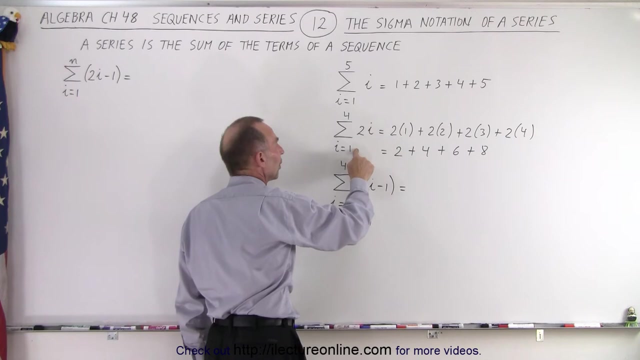 because that's the upper limit, And each time we multiply times two, So two times one plus two plus three plus two times four or two plus four plus six plus eight, And that is the series that can be compactly written like this. So it's two times the number i when i goes from one to four. 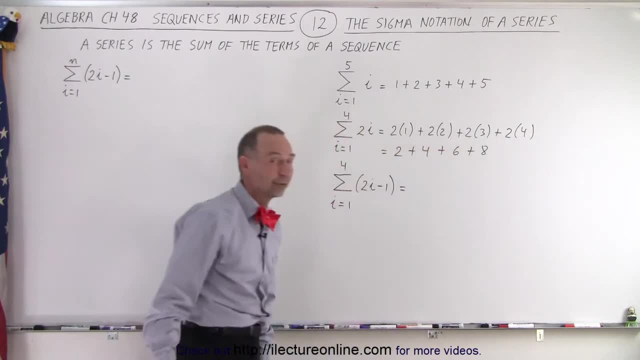 and this means we're going to sum them all up. That's why we add up all those terms. What if we get something like this: Now let's do this one together, So we have the sum from i going from one to four of two. i minus one. So we're going to let i go from one to two to three. 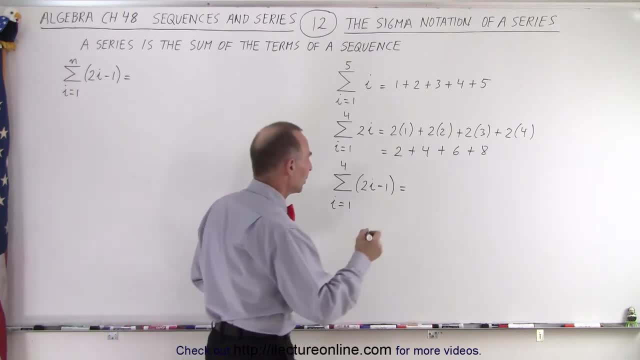 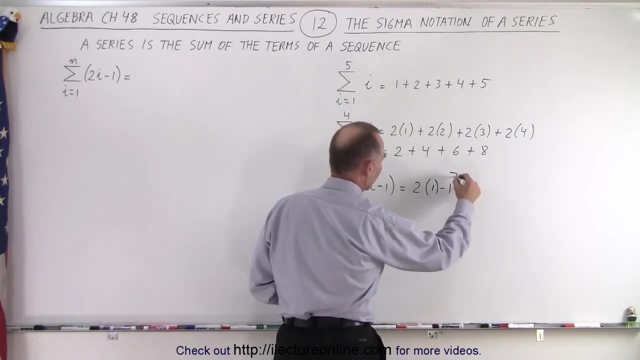 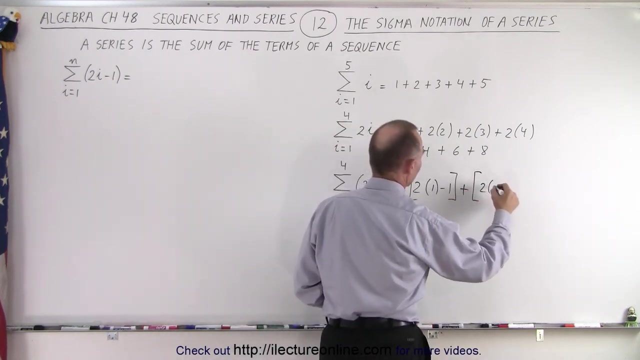 and we just plug in for i each single time and add them all up. So this becomes two times i, which is starting at one minus one plus, and I'll put brackets around it. so that's the first term plus now let i equals two, So we have two times two minus one. So two times two minus one. 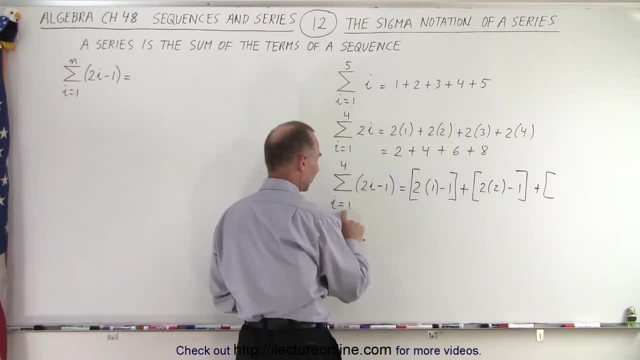 plus. now we have two times the next value for i, which is three. So two times three, 1 and on. finally, we have the next and the last value for i: 2 times 4 minus 1. so 2 times 4 minus. 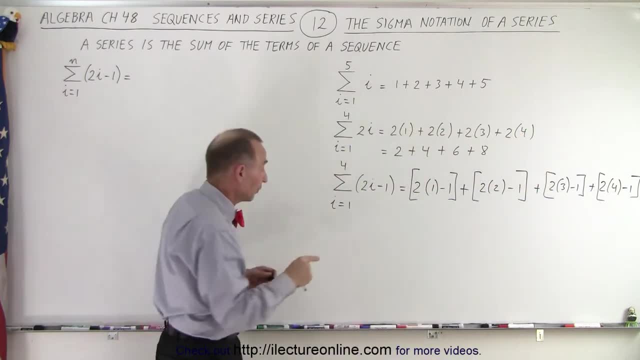 1. so here are the four terms. why do we know there's four terms? because i goes from 1 to 4, so we have: i equals 1, i equals 2, i equals 3, i equals 4. this means we sum them all up and this is what. 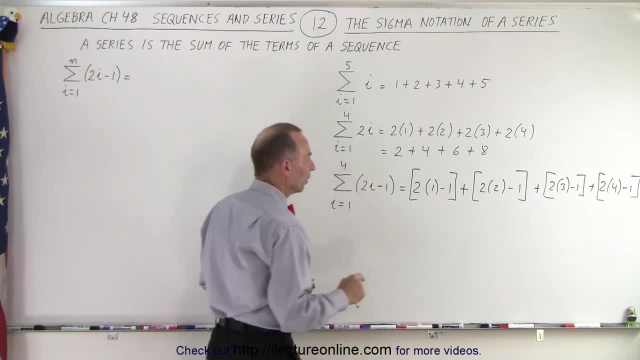 we're summing 2 times i as i goes from 1 to 4 minus 1, so 2 times 1 minus 1, 2 times 2 minus 1, 2 times 3 minus 1, 2 times 4 minus 1, and that is what we mean by that sigma notation. well, let's. 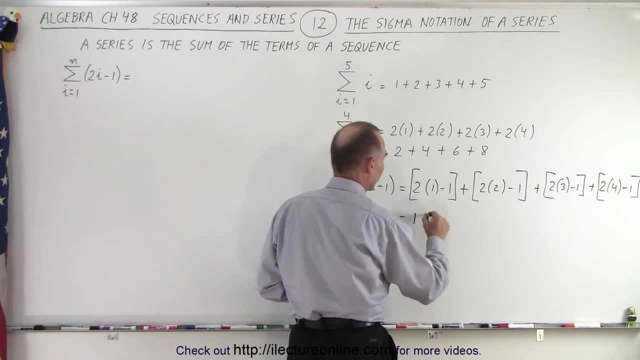 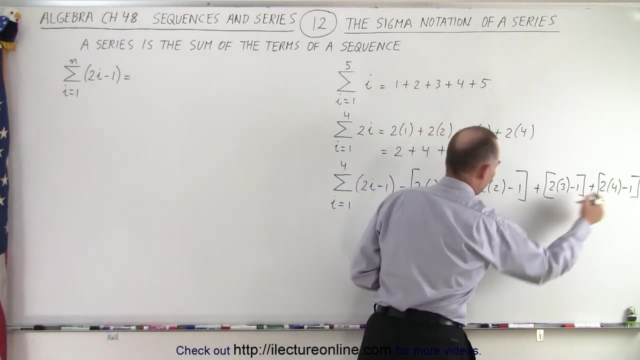 finish it up. so this is equal to 2 minus 1, which is 1 plus 4 minus 1, which is 3, plus 6 minus 1, which is 5 plus 8 minus 1, which is 7. so that would then be the series and the result of the series. 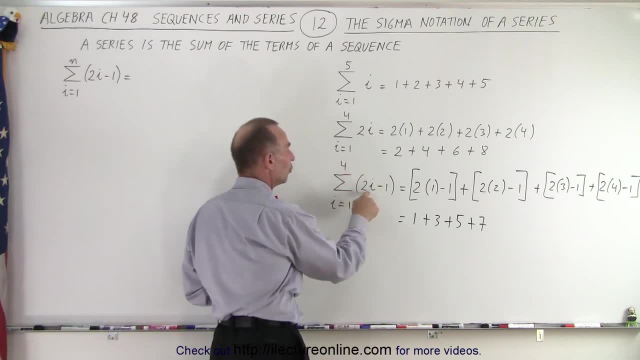 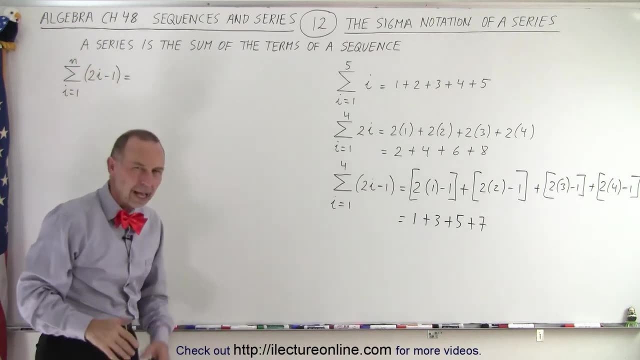 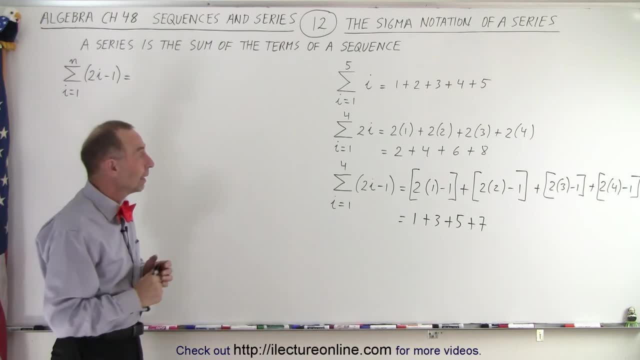 number, any value for i, any integer. it can be anything. so what we're going to do here is we're going to plug that in and at the very last term, we replace i with an n instead of a number. so this is how it goes. so this would be 2 times 1 minus, 1 plus, and looks exactly the same as that: 2 times.